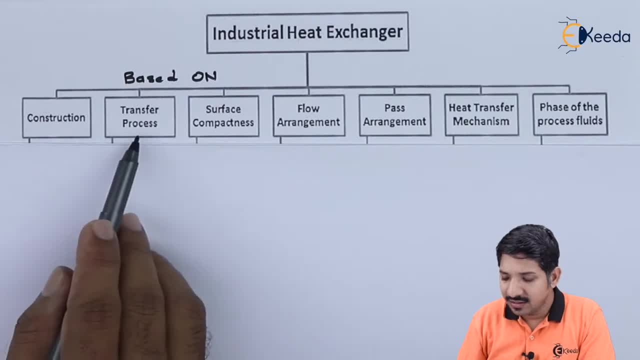 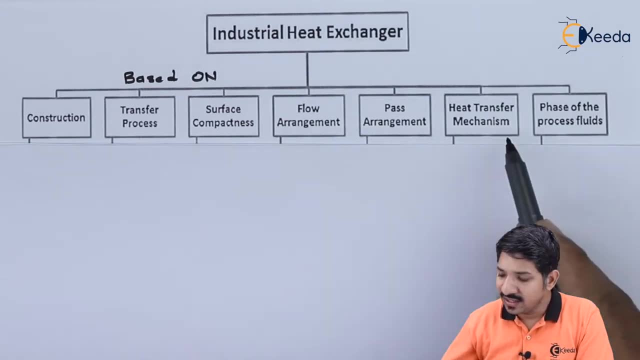 are there, such as based on construction, then the transfer process, then the surface compactness flow arrangement, then the pass arrangement, Then the mechanism and then the phases of fluid. Obviously, the phases of fluid, it can be liquid or gaseous- Then, based on mechanism, we have either based on evaporator or condenser. 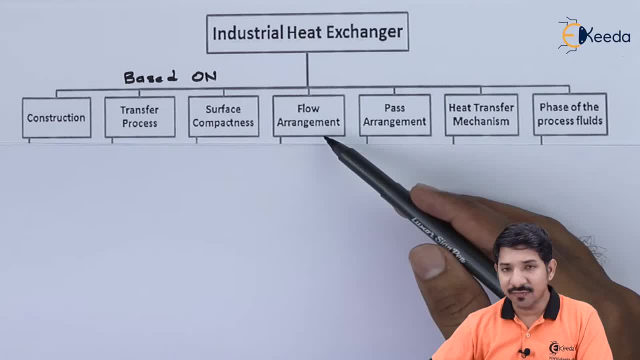 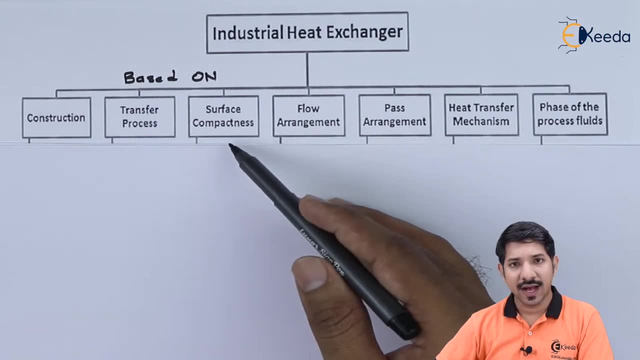 Then based on passes, it can be a single pass or double pass. Then flow arrangement: obviously we have parallel flow, counter flow and cross flow arrangement. Surface compactness: either it can be a very compact heat exchanger or a very lean heat exchanger. 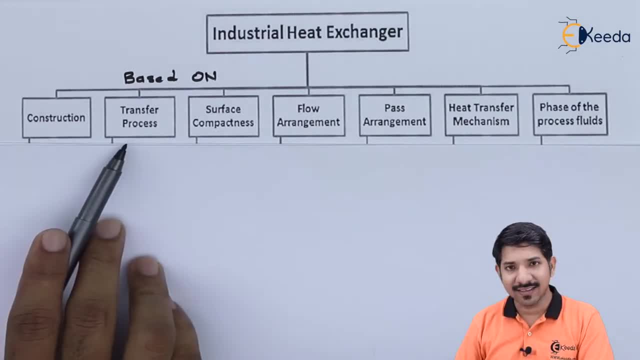 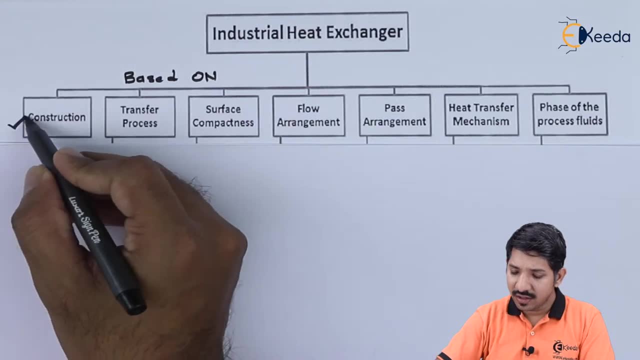 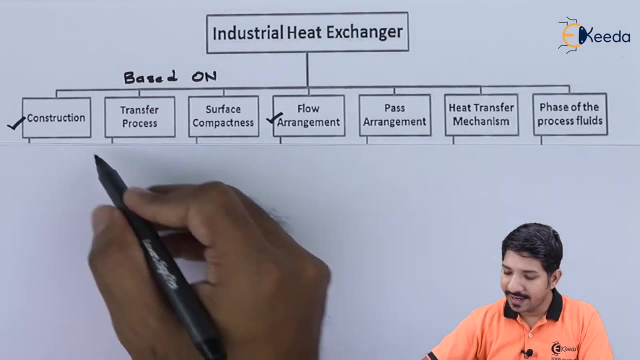 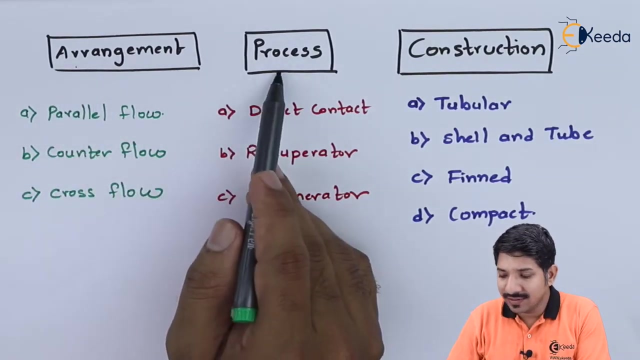 Then the transfer process, Again based on process- also, it can be classified- and based on construction. So out of all these three, we are going to focus on construction, flow, arrangement and the process itself, As I have said before, based on the arrangement, then process and construction. So, as per the 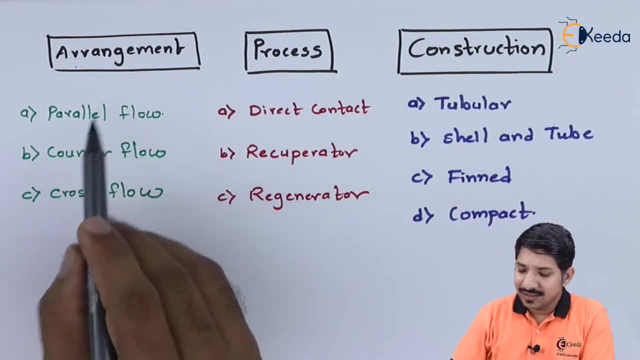 academics. Chapter 4, Chapter 5, spar 1, 10erschaftungs hologram- DAVID BROGDON GmbH. Part. Part 2, the analysis based. these three are the most important parameter on which the heat exchanger. 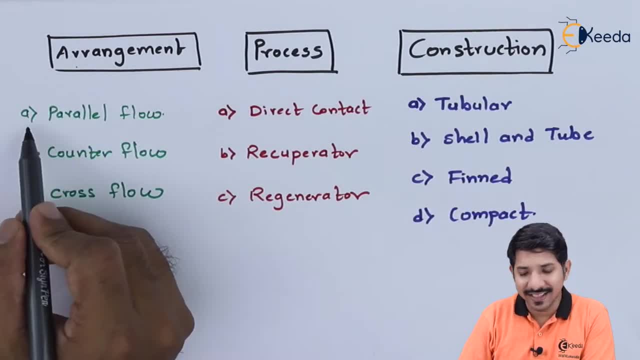 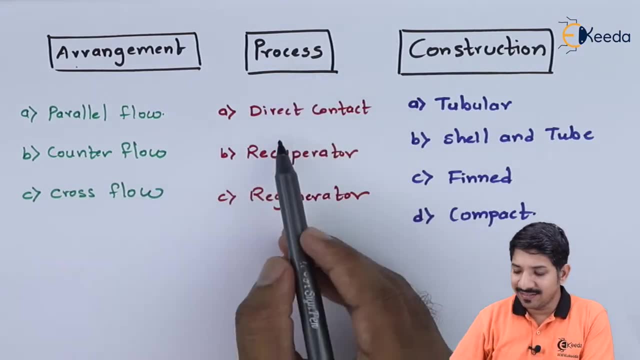 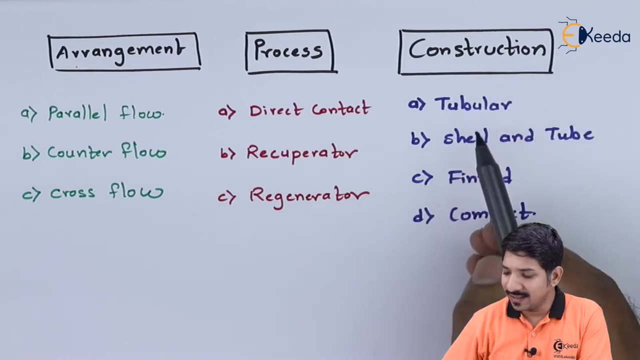 must be classified. so, based on arrangement, it can be classified in three ways. one is parallel flow, counter flow and cross flow. based on process, it can be classified as direct contact, recuperator and regenerator. and then, based on construction, it can be classified in the four ways. one is tubular. 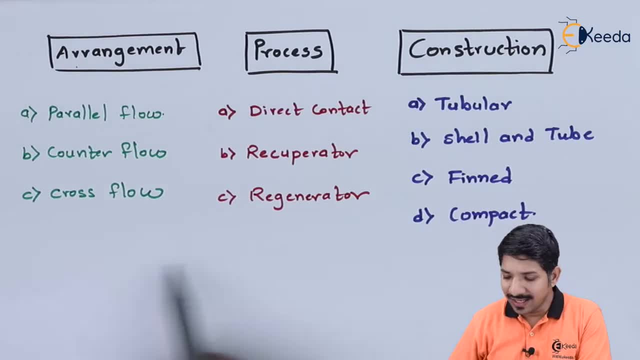 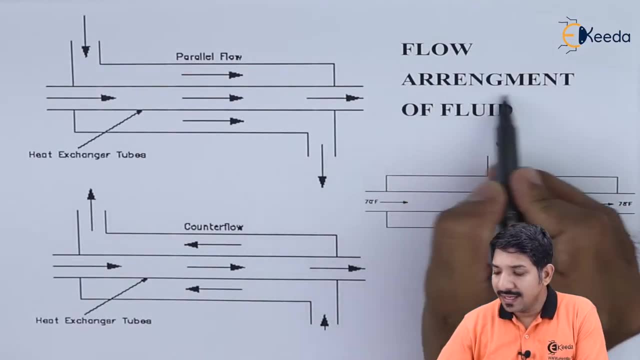 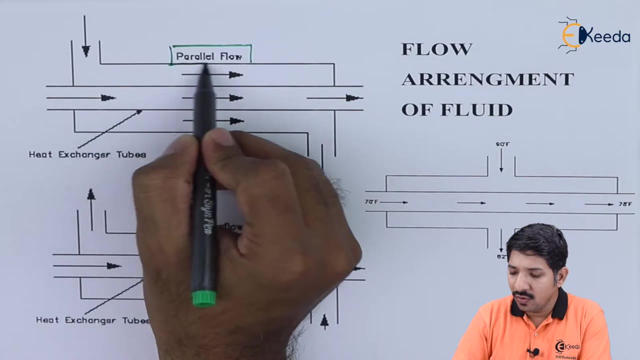 shell and tube, fin and compact. now let us look at all these individual heat exchangers one by one. now here we have considered based on the flow arrangement. so, based on flow arrangement, as we have said before, that it can be classified as parallel flow, counter flow or the cross flow. 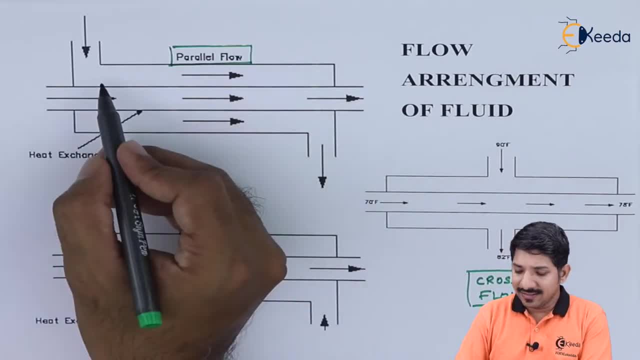 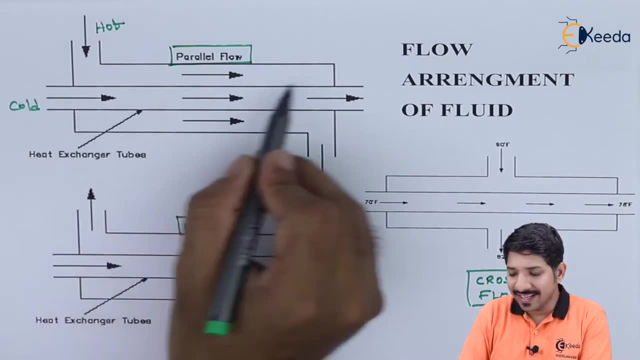 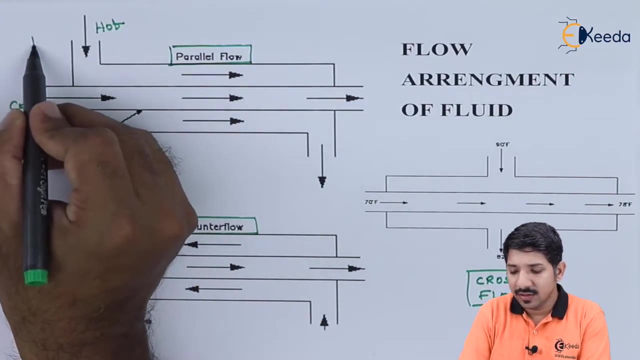 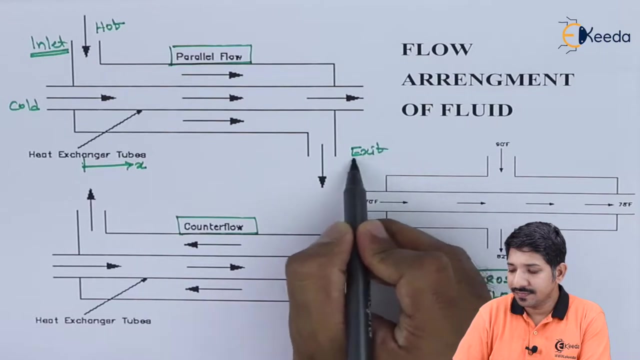 so what do you mean by the parallel flow? parallel flow is the case where the hot fluid and the cold fluid, they travel in the same direction. so if i say that this is my x direction, this is my entry, or the inlet and this is my exit, then we can say that the hot and cold fluid will travel. 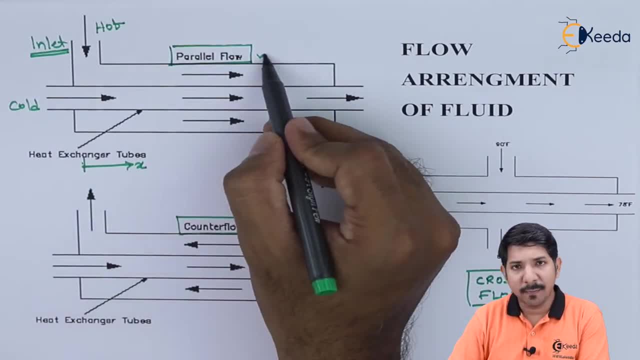 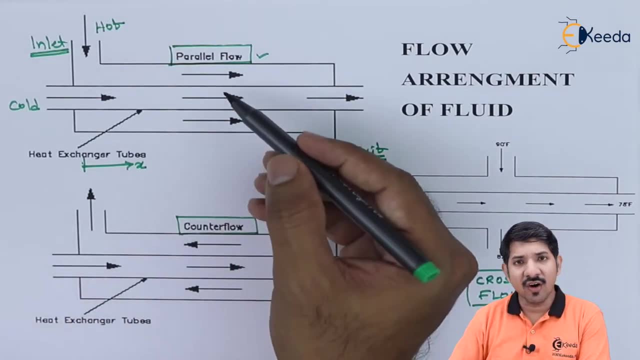 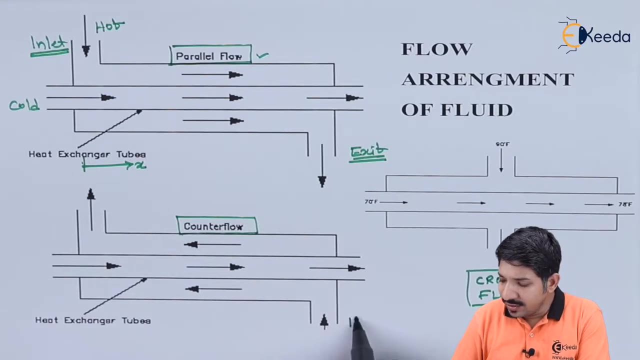 in the same direction. so that is all about the parallel flow. similarly, in case of a counter flow, obviously we will have a ulta of what we have in a parallel flow. so if the flow, that is, let's say, a hot fluid, let's say this is the inlet of hot fluid, then the inlet of cold field will be. 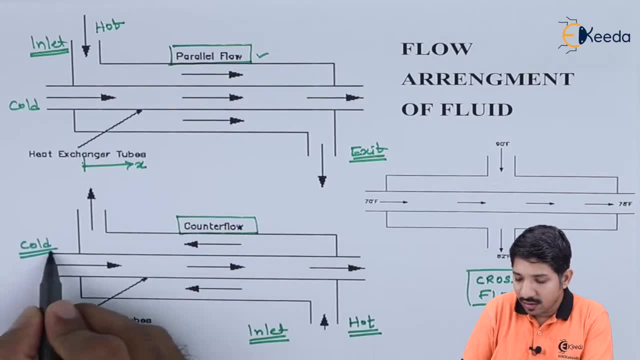 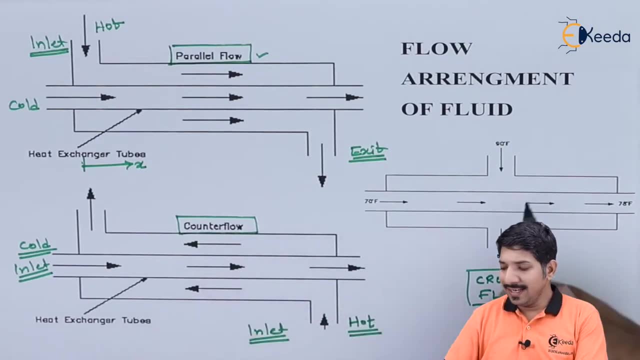 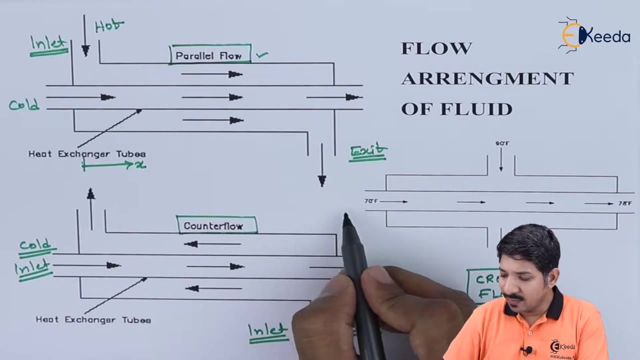 exactly in opposite direction. so in this way, basically, we will get to have a counter type of flow and in case of a cross flow, obviously the direction of the flow will be perpendicular to each other. if suppose the hot fluid is traveling in this direction, then the cold fluid will travel in the exactly 90 degree celsius to 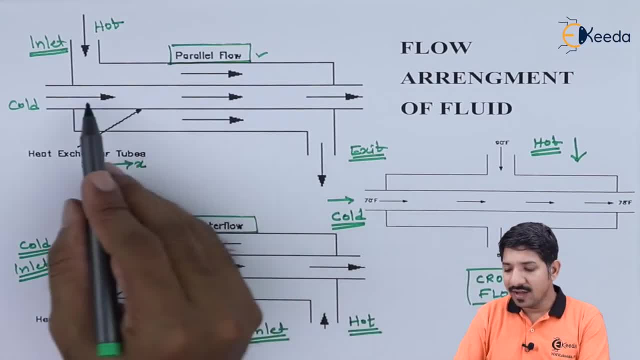 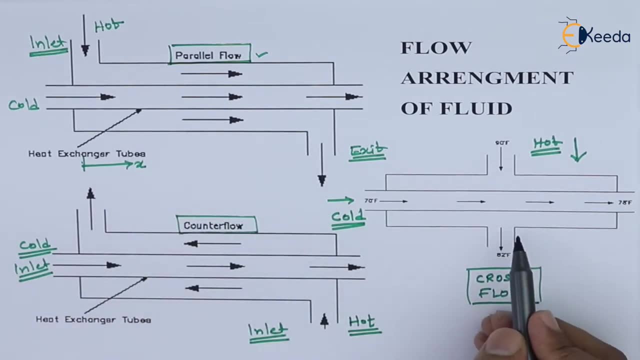 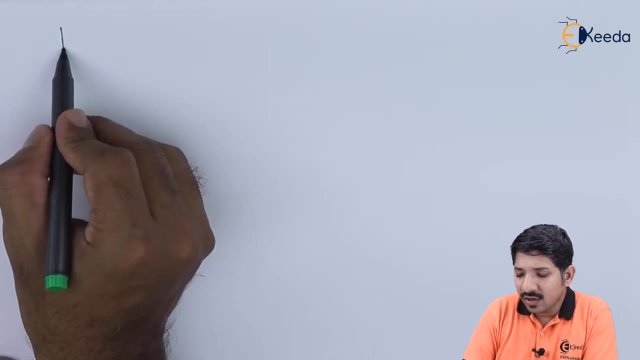 the that of the hot fluid. so here we have got zero degree celsius between the hot and cold fluid, here literally 180 degree celsius difference, and here 90 degree celsius, and here 90 degree celsius difference. again based on that, we can draw. 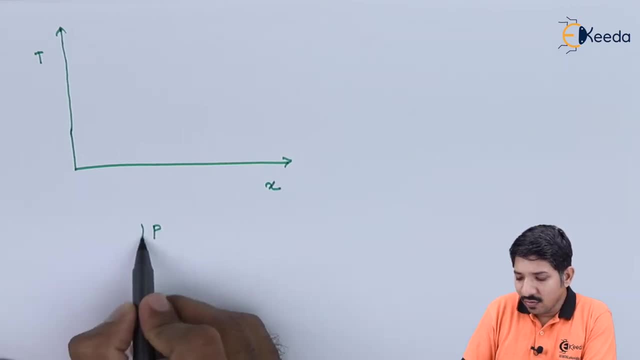 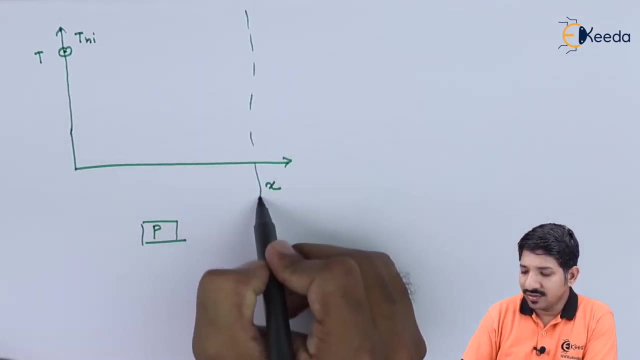 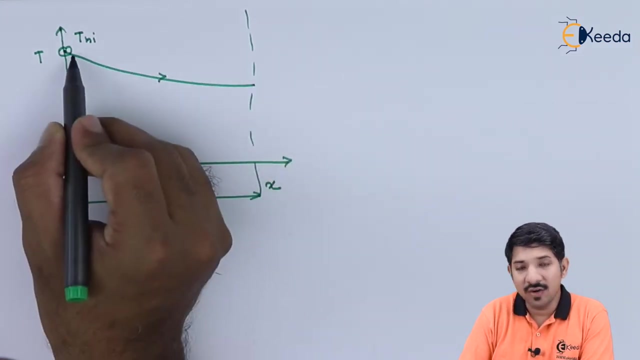 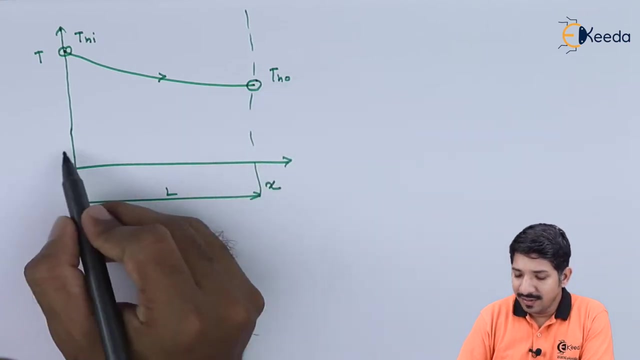 temperature versus x diagram. if it is a parallel flow, then this can be considered as thi. if suppose this is the length, then the hot fluid will keep on eliminating heat and the temperature will decrease to, let's say, th o. similarly, the cold fluid will start from here. so this is, let's say, tsi is the inlet. 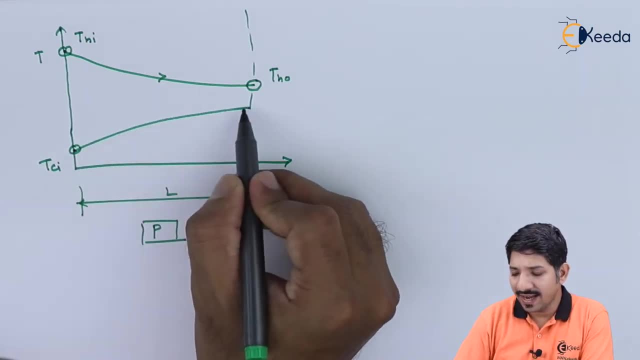 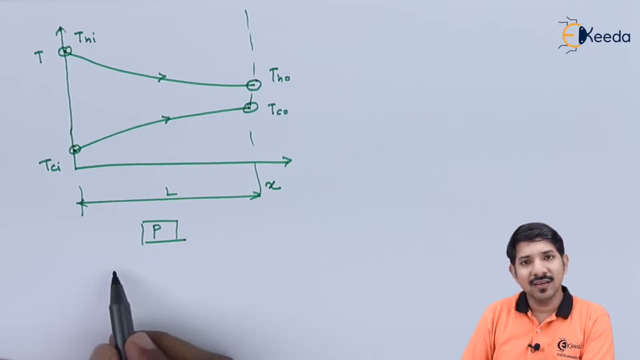 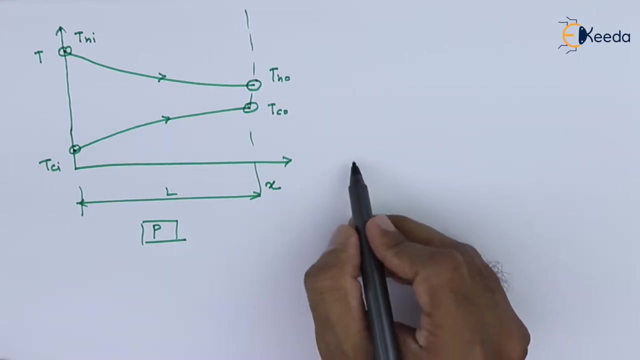 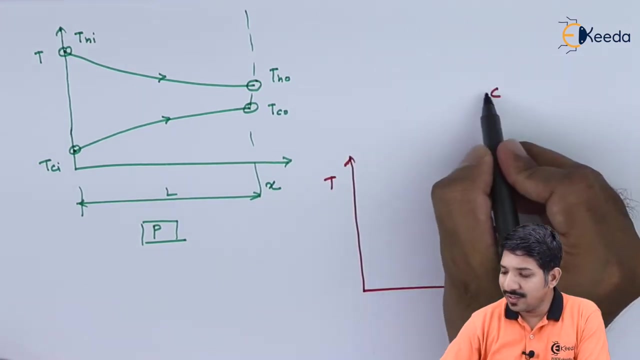 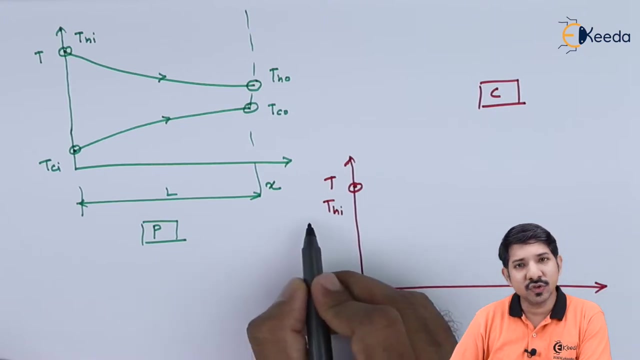 temperature of cold fluid and it will gain the temperature and the heat to reach the tco temperature. so this can be said as the tx diagram for the parallel flow heat exchanger. similarly we can draw a tx diagram for the counter flow heat exchanger for the hot fluid. again, let us say thi is the inlet temperature of hot fluid. let's say this: 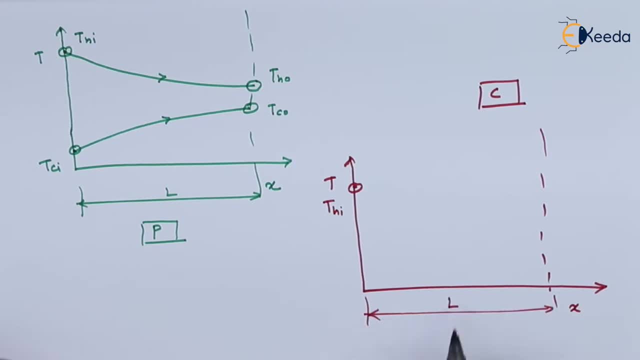 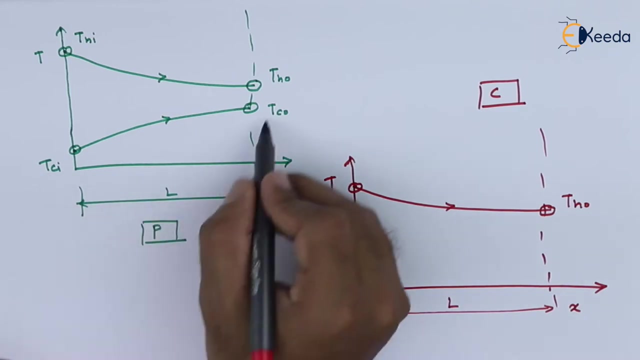 is the total length of the heat exchanger, which is l. so obviously the temperature by the hot fluid is decreasing. so the inlet temperature is thi, which is the highest temperature, and it is decreased to, let's say, t ho. but in case of a cold fluid we will have a counter flow here, so the cold fluid will. 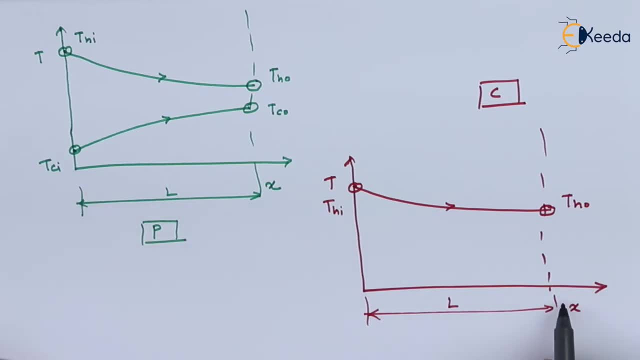 not start from x equal to zero, but it will start from x equal to l. so let us say it will start somewhere from here. so this will become tci, that is the inlet temperature of cold fluid, and again it will keep on getting the heat to, let's say, reach somewhere. here. this is become my tco. 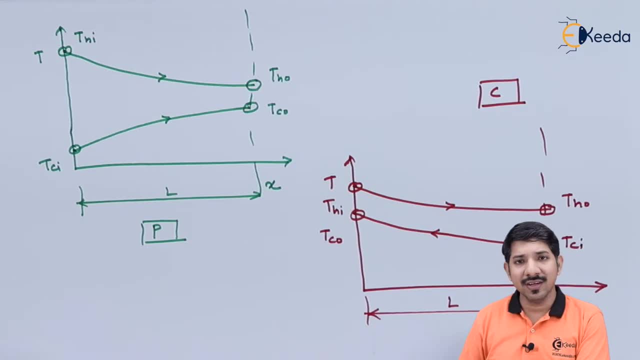 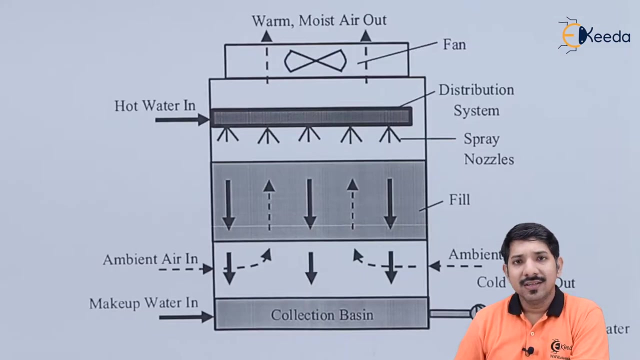 so this can be said as the temperature versus the length diagram for the parallel and the counter flow. we will see all these two diagrams later for the sake of analysis now. next, we are going to talk about the direct contact recuperator and regenerator. this one is the direct contact. 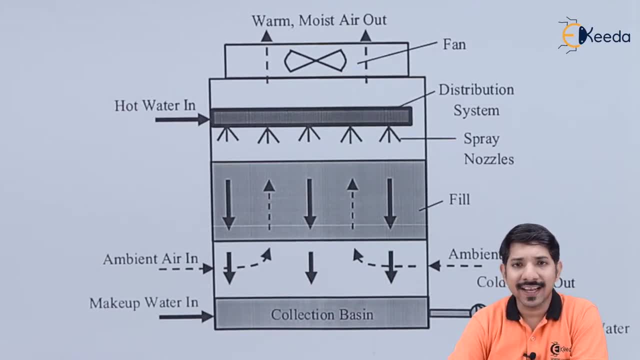 heat exchanger, as i have said before, in case of a direct contact, by the name itself, we can say that in case of a direct contact heat exchanger, the hot and cold fluid will mix with each other. the best example for the direct type heat exchanger is nothing but the cooling tower. 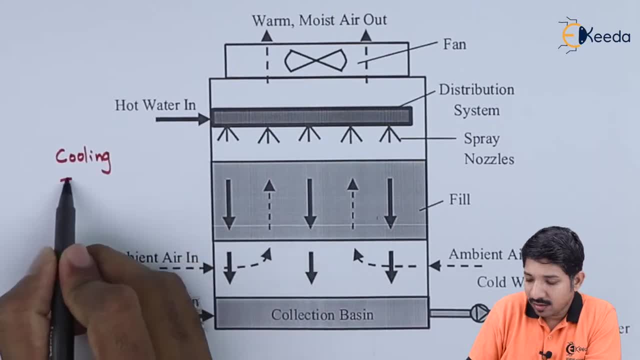 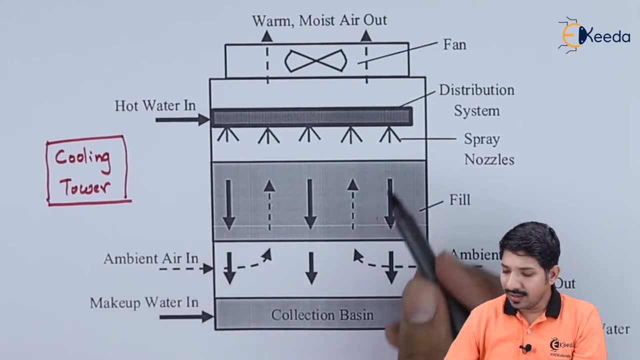 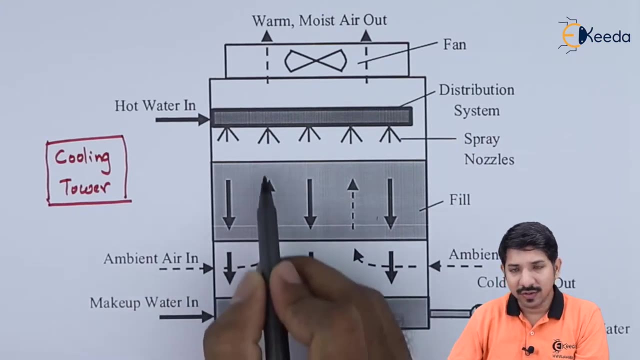 so this is the example of cooling tower. so this is the example of cooling tower. now let us understand. what do we have in a cooling tower? the air will get entered from this area here you, There will be a blower over here and the same air will enter from both the side in the upward 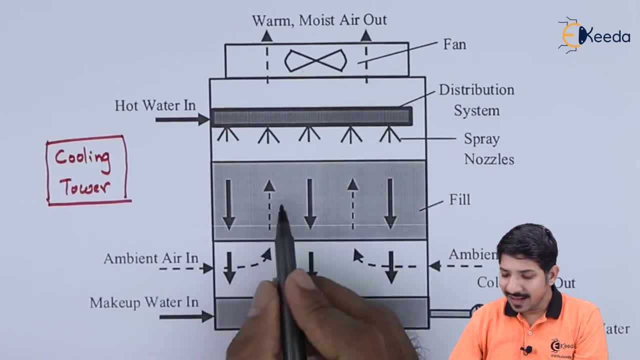 direction, So there is a upward movement of the air and then a hot water will get flown from here. So basically, here the heat exchange will takes place from the small water droplet of a hot water and that of the air. So this way we will get a moist or warm air at the outlet of the cooling tower. 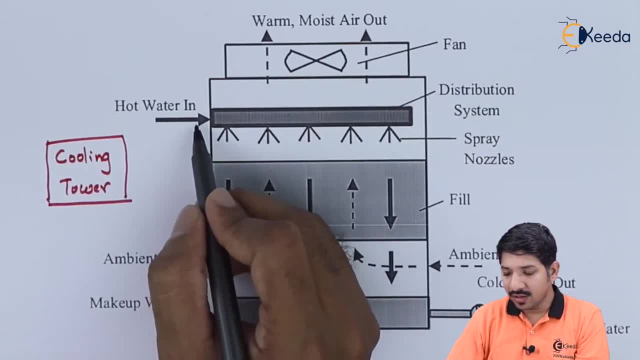 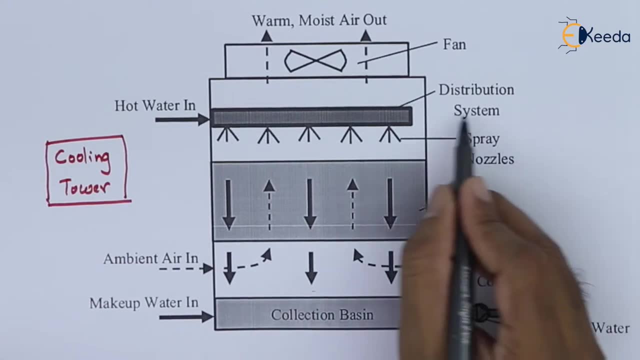 This way. here we have a collection of basins, So the whatever water droplets which we are pouring from the upside will come down and will get collected over here, and the same will be sent in the upward direction. So why is it called a direct contact? 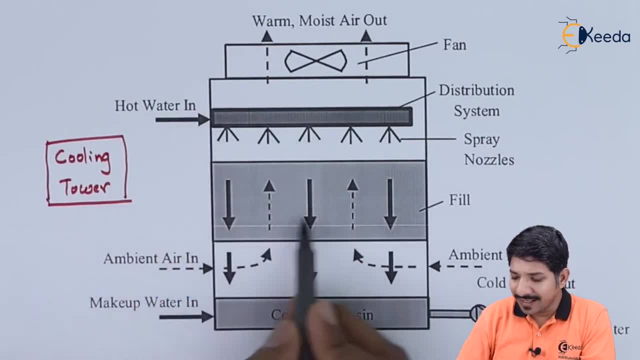 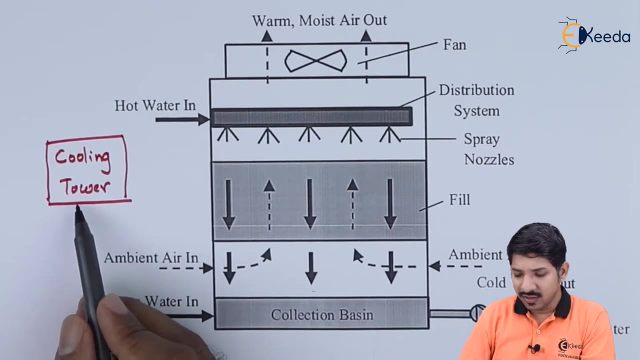 Because here the heat exchange takes place between the water droplets and the ambient air directly. There is no metal as such in between. The heat transfer is direct in this case. So such type of heat exchanger widely available. It is widely used in many industries. 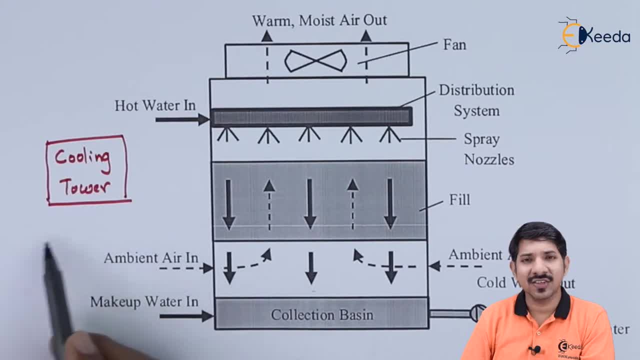 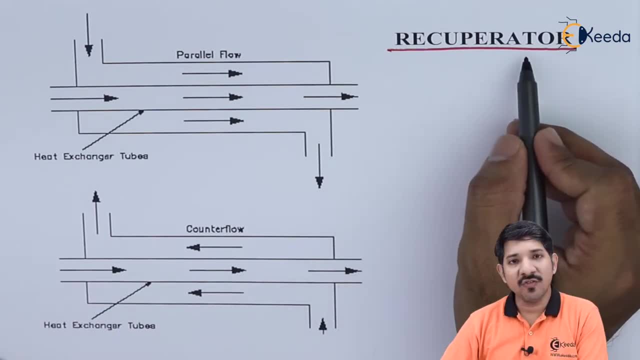 So cooling tower is also used in many industries, such as refrigeration industries or in a power sectors. Next one is recuperator. Now, what do you mean by recuperator? Recuperator is a type of heat exchanger where the heat transfer takes place in such a way. 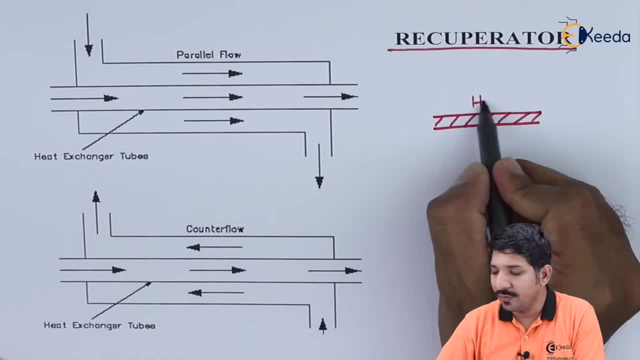 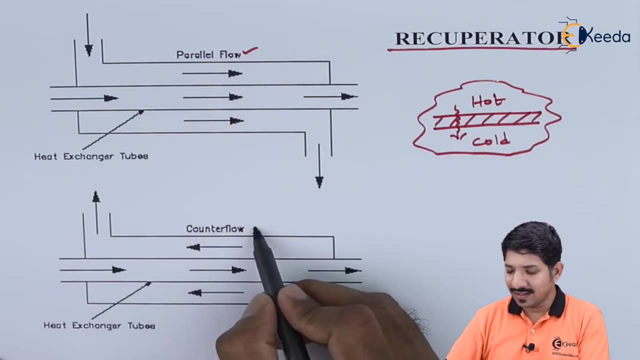 that a small metal piece will be there between the hot fluid and a cold fluid, So heat transfer will obviously takes place through this metal rod. So this is the heat transfer. So again, this kind of example can be seen in case of a parallel flow as well as a counter. 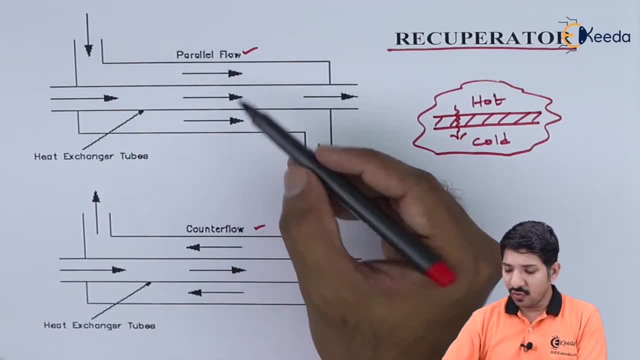 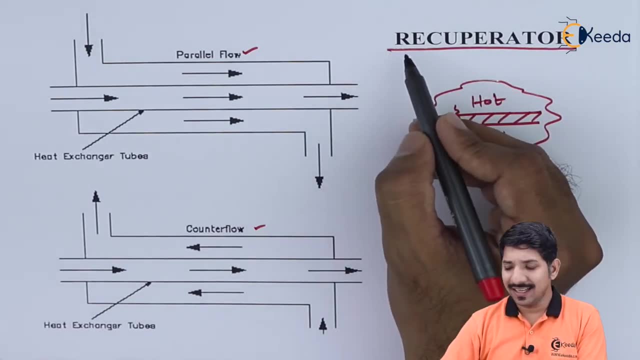 flow and a cross flow heat exchanger. So this parallel flow, counter flow and cross flow heat exchangers are nothing but the recuperator heat exchanger, Mostly in industry. we generally you will find that this kind of heat exchanger widely used in many applications. 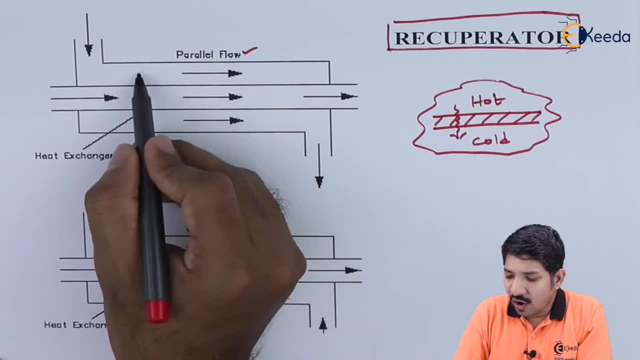 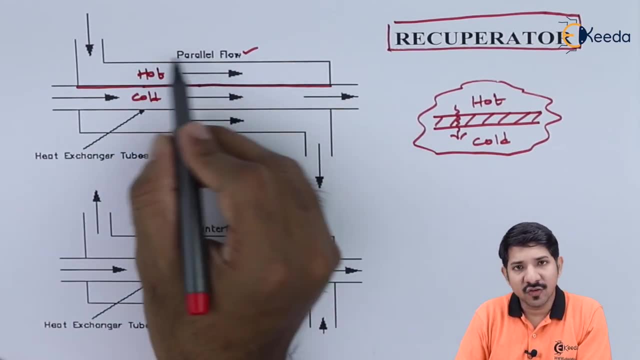 Here also, you can see that in case of a hot and cold fluid, we only have a small plate. Here also you can see that in case of a hot and cold fluid, we only have a small plate In case of a parallel flow. so is the case with a counter flow. 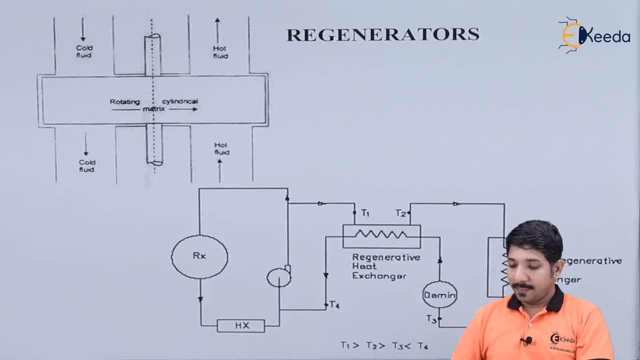 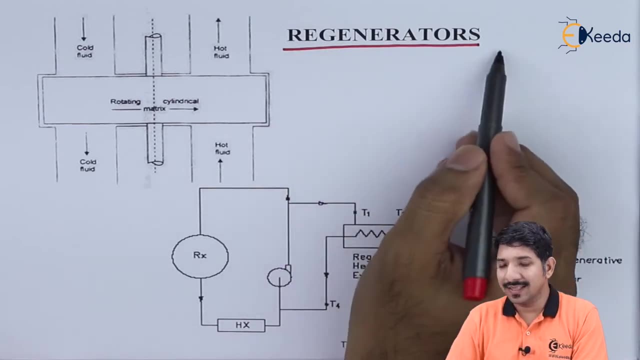 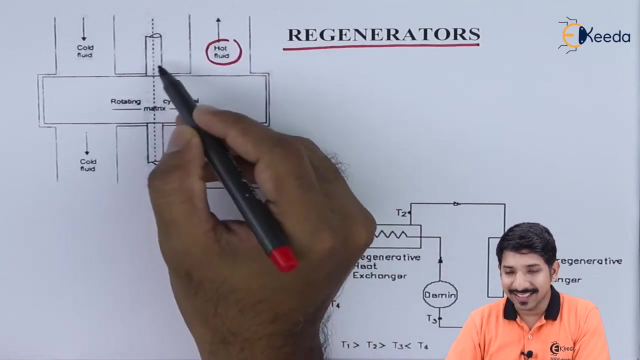 That is why we can call this as a recuperator, heat exchanger. And then the last one in this category is regenerator. Now again, let us try and understand. what do you mean by the regenerator. Regenerator is a heat exchanger where a hot fluid will be passed through some passage. 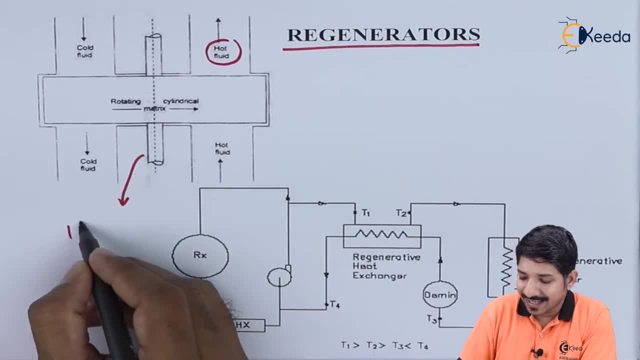 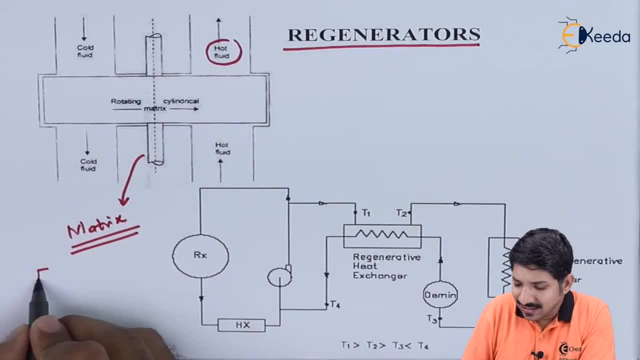 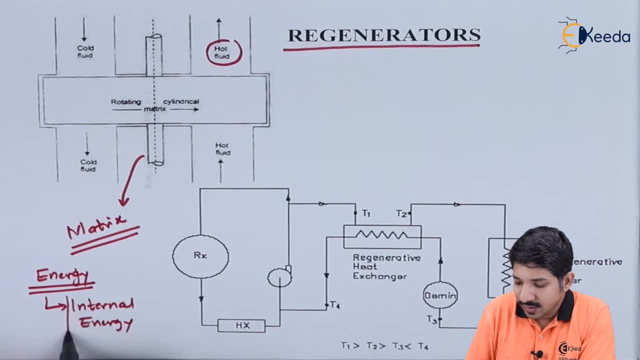 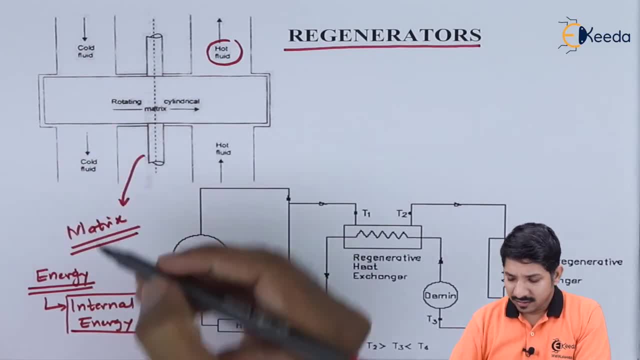 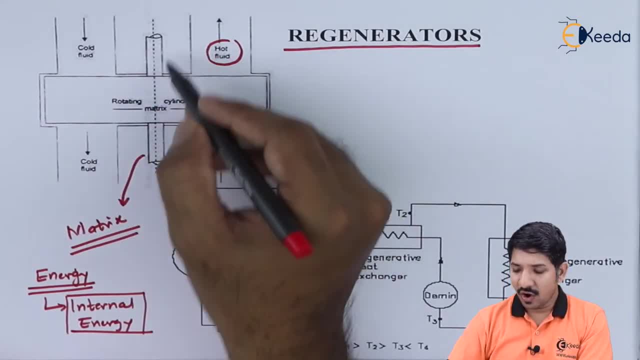 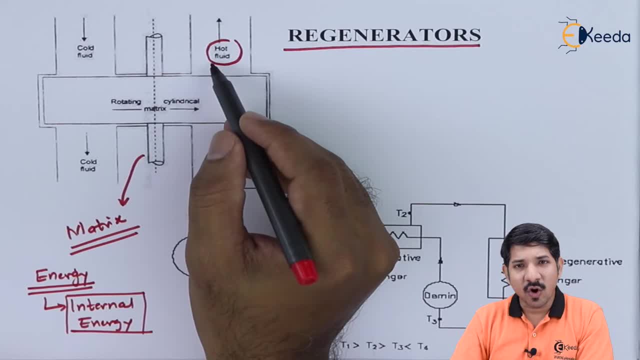 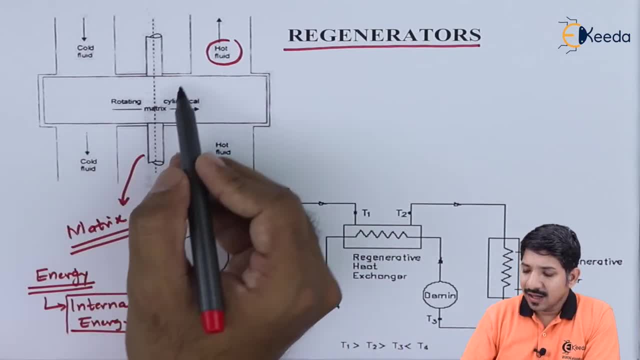 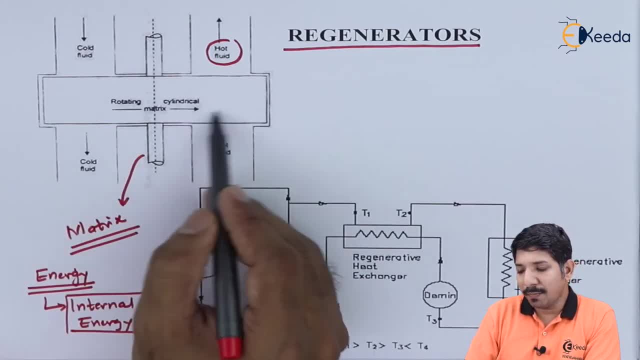 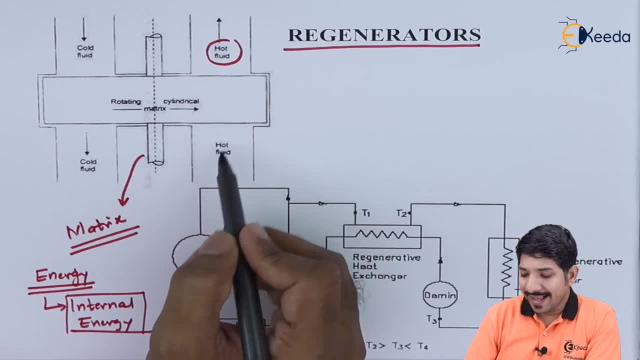 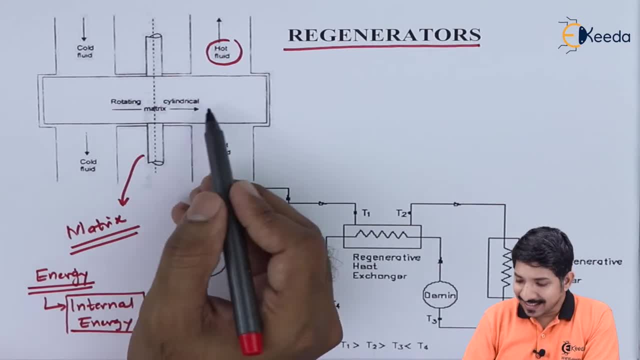 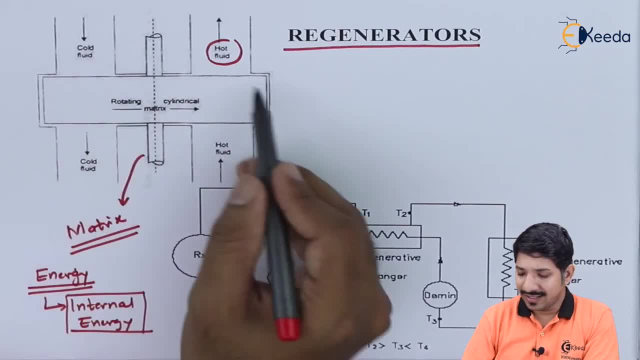 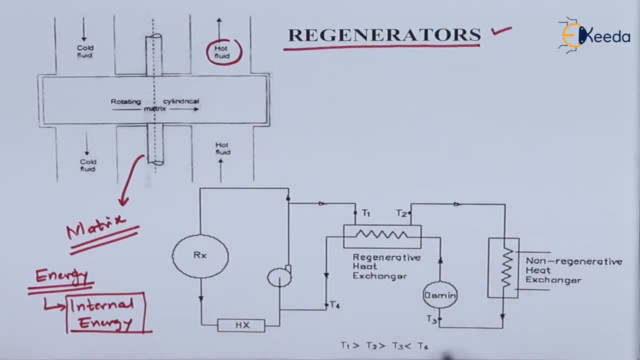 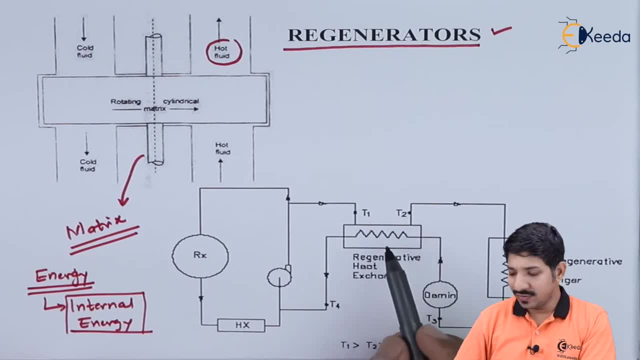 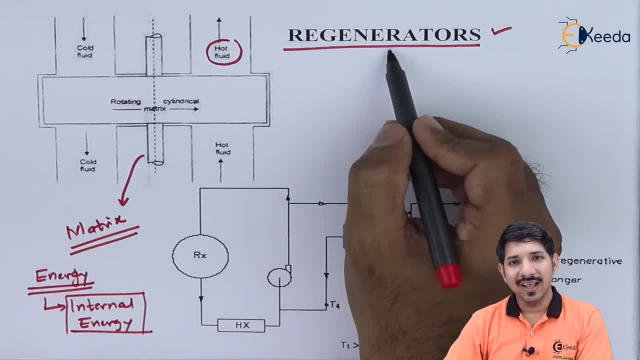 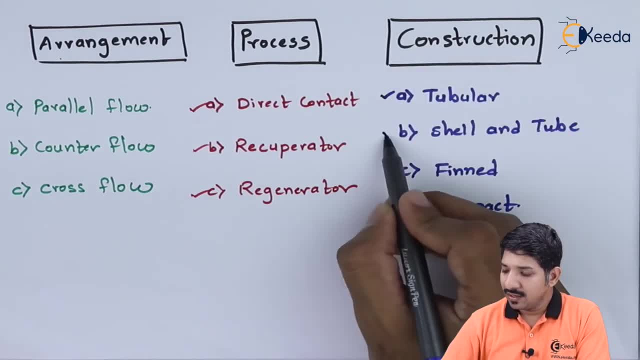 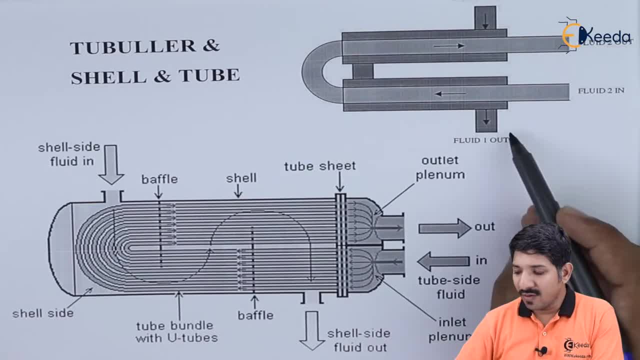 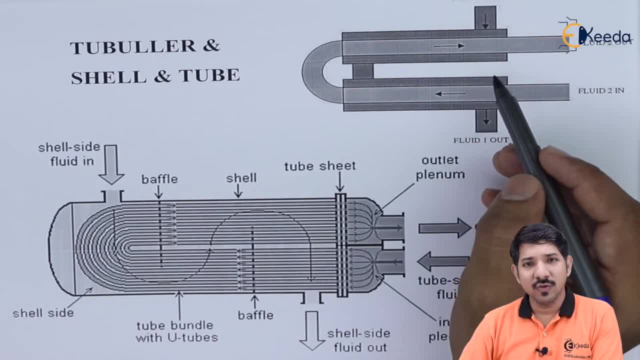 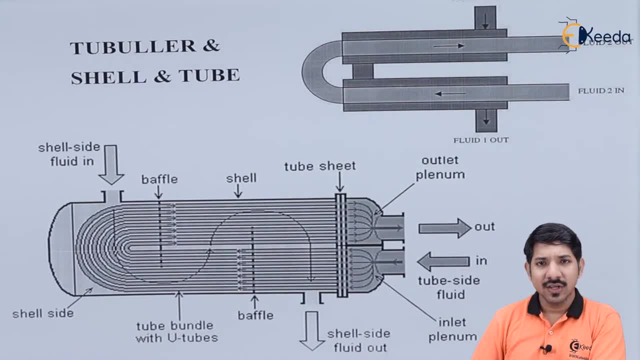 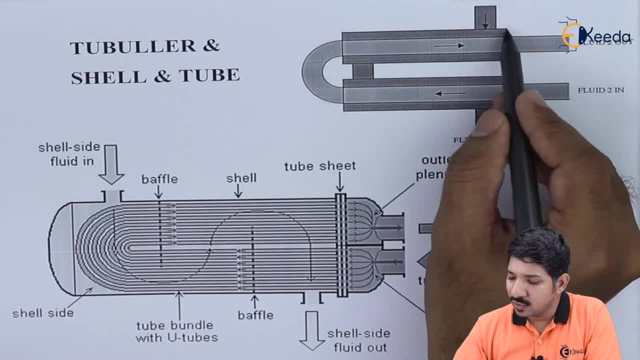 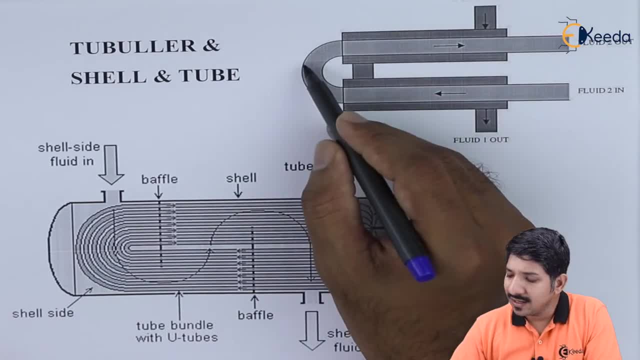 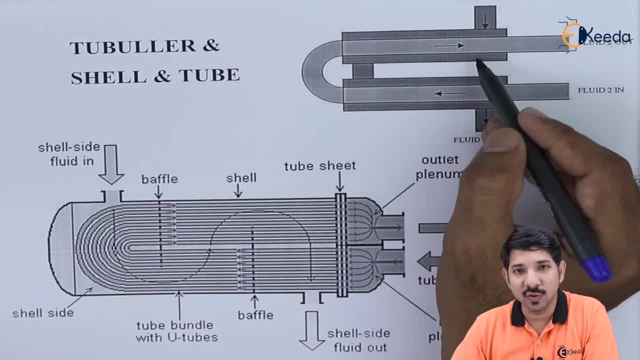 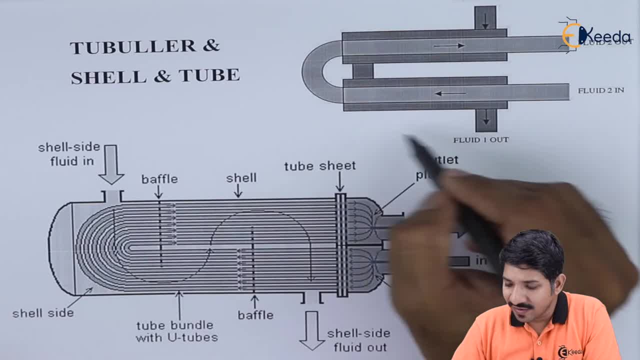 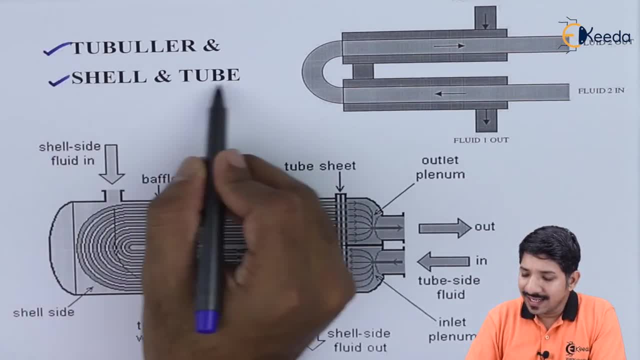 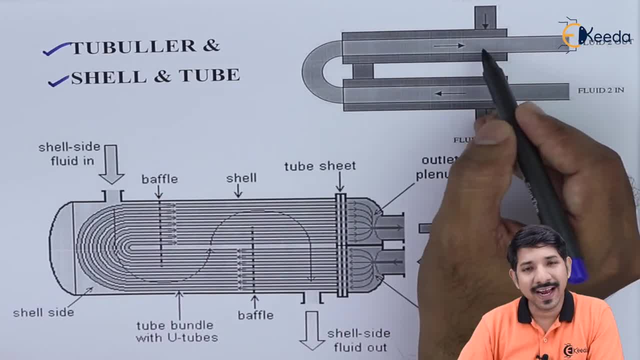 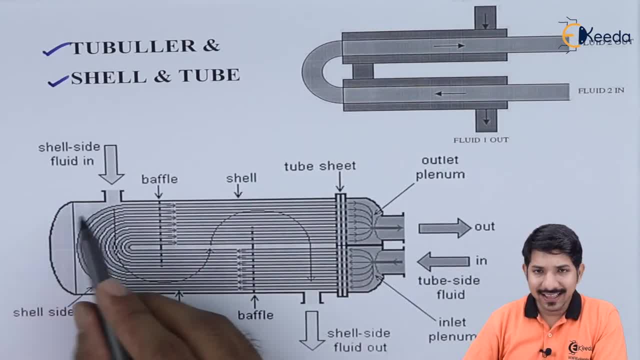 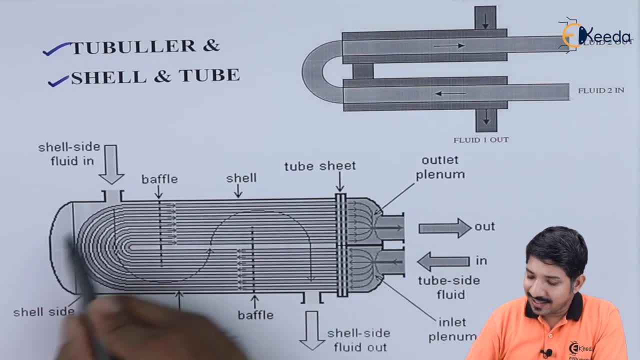 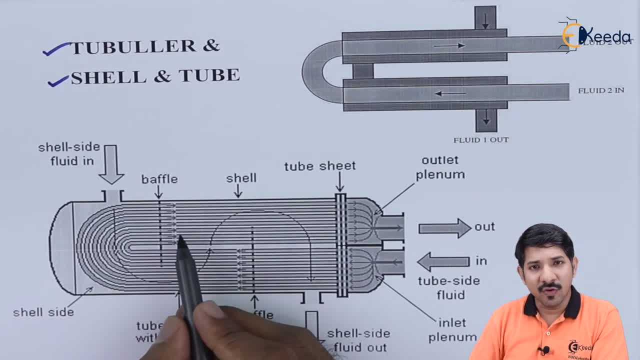 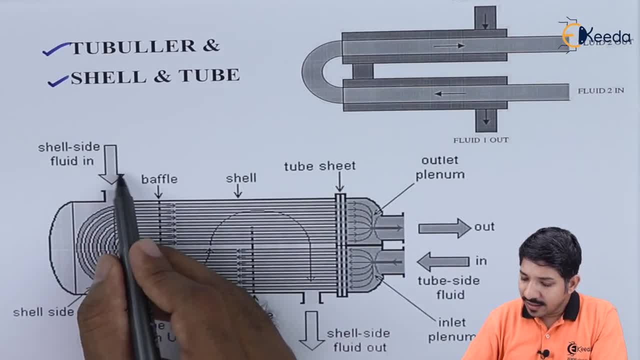 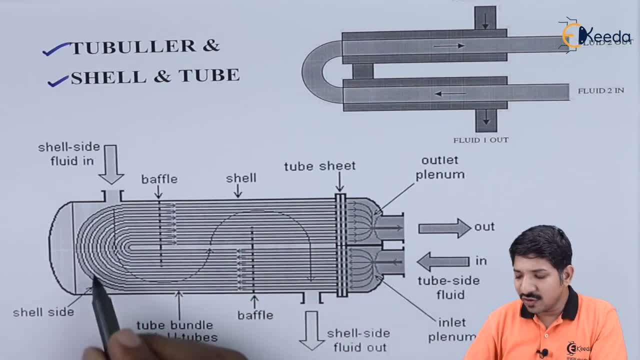 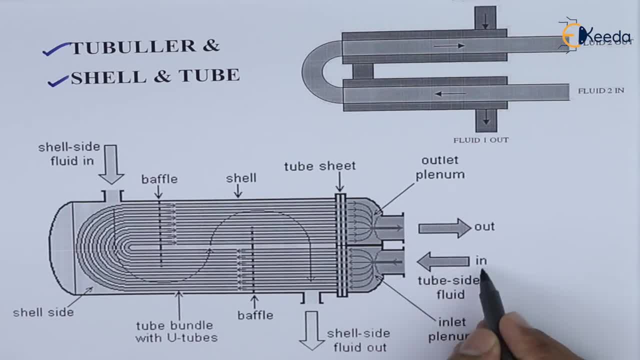 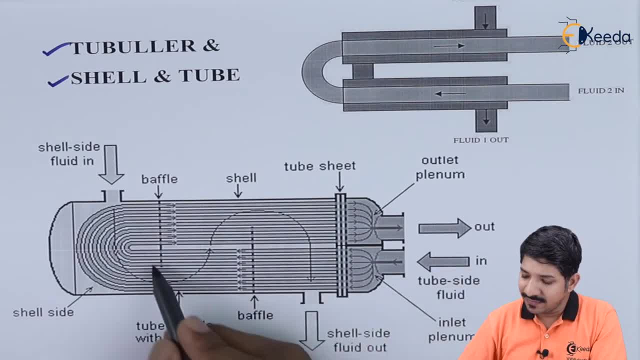 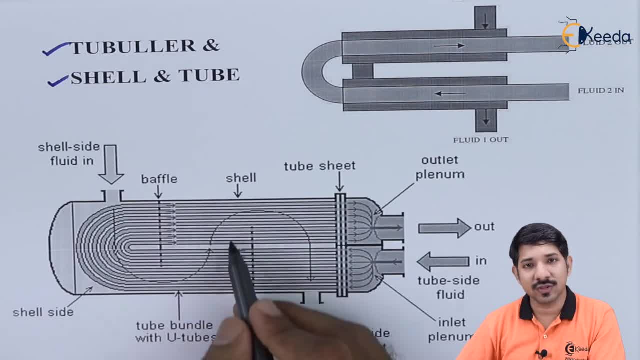 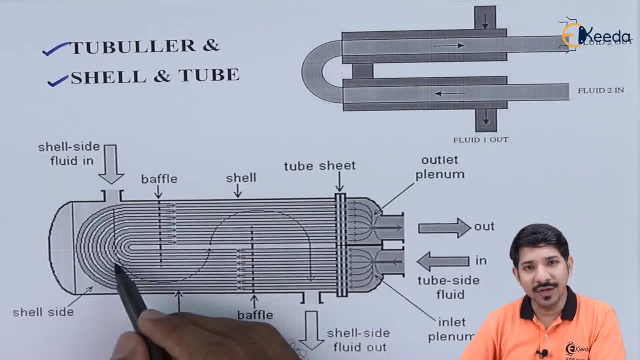 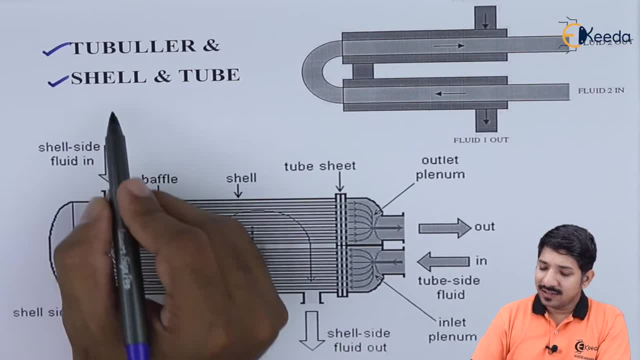 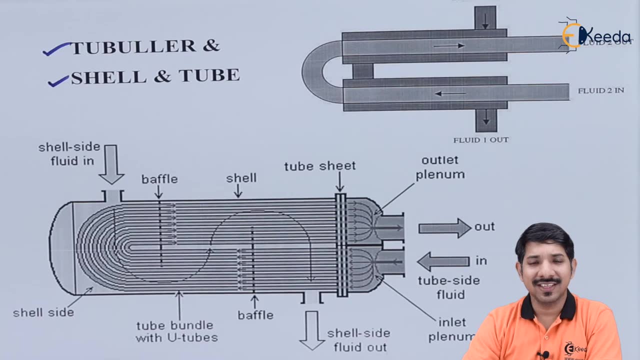 That passage is mostly called as matrix. Now what is that passage called? That passage is mostly called as matrix. Now what is that passage called? tube type of heat exchangers are widely used in the industry, so mostly the domestic heat exchangers such as the water heater. they are this type of only where they will use shell and tube. 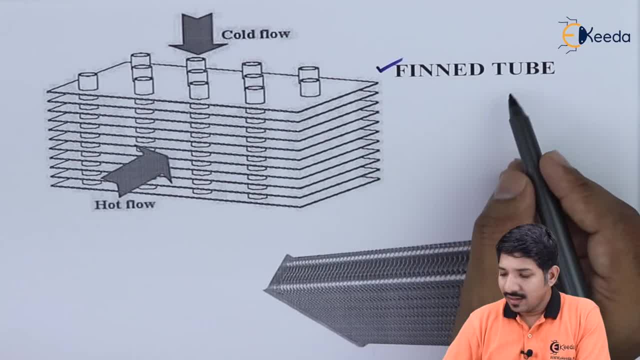 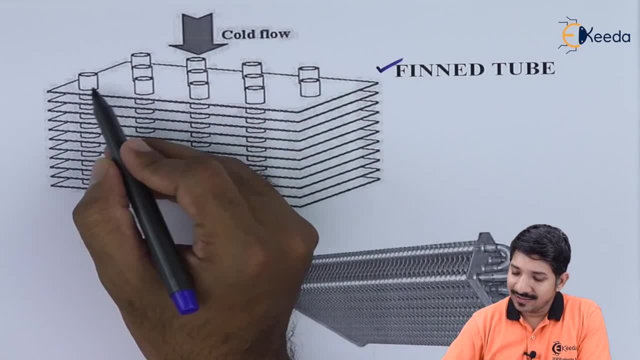 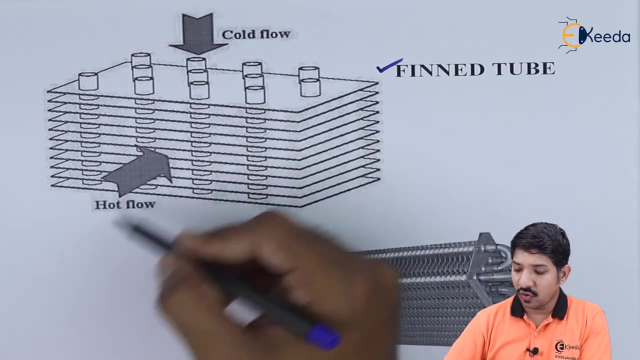 type of arrangement itself. next one is a fin tube. as we can see from the diagram, in case of a fin tube, let's say, the cold fluid is passing through the tubes. so these are my tubes here, number of tubes which are arranged in this manner- and then the cold fluid will pass with the cross flow and 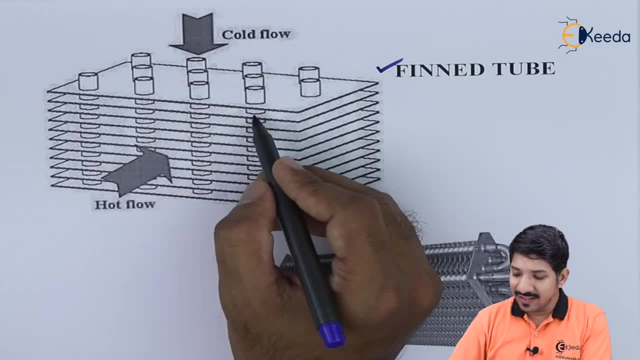 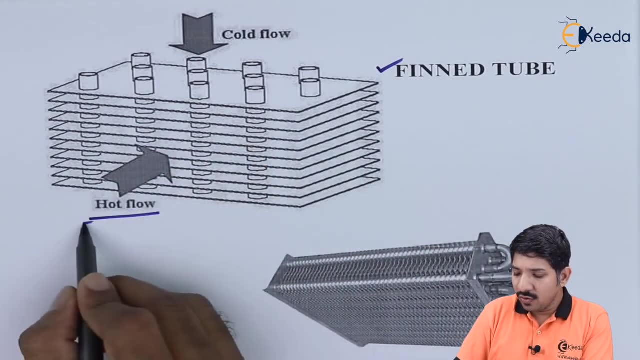 then there will be fins around the tube, so this fin will basically enhance the heat transfer rate. so this type of heat exchanger used when the hot flow is in the form of gases. for the gases the value of h is quite less as compared to that of liquid.